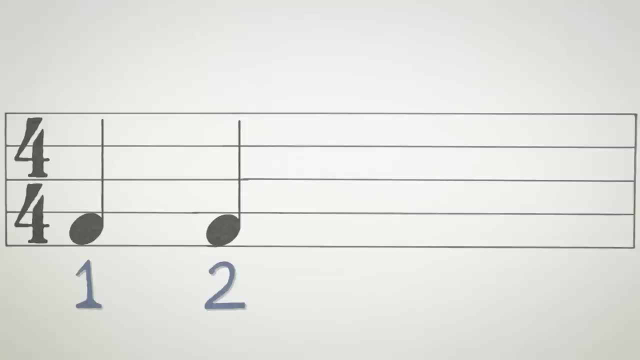 keep track of different rhythms. As we said before in 4-4 time quarter notes. last one beat. so we just count them on the beat as one, two, three, four. One two, three, four, Eighth notes. however, only last half a beat. 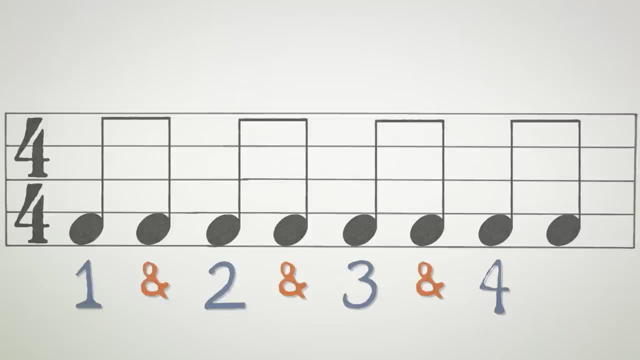 so we need to add an and between the beats to track them. So we count one and two and three and four, and one and two and three and four and 16th notes have four notes per beat. 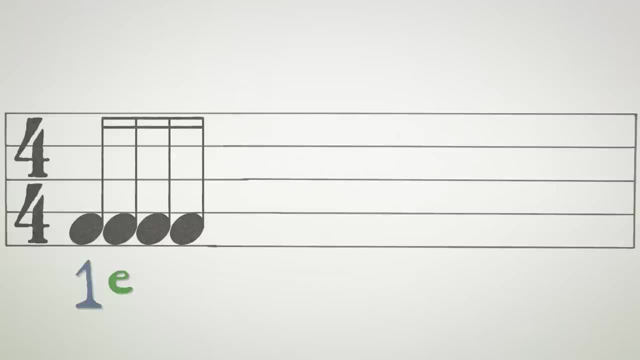 One E and a two E and a three E and a four E and a one E and a two E and a three E and a four E and a, And with triplets we count them as one triplet, two triplet, three triplet, four triplet. 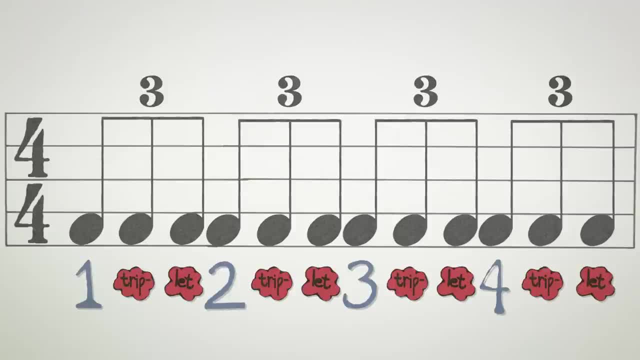 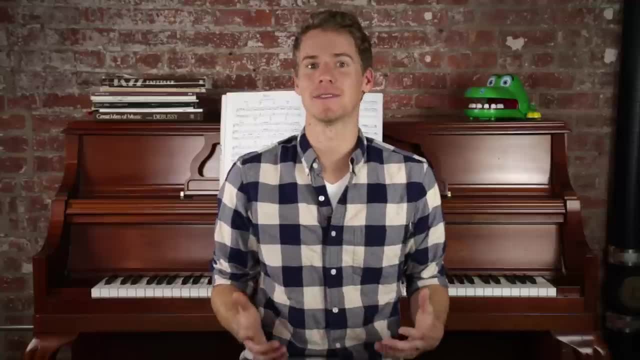 one triplet, two triplet, three triplet, four triplet. This is where clapping really helps us, because we have to keep track of both the beat and the rhythm at the same time. So what I like to do is clap and say the actual rhythm we're playing. 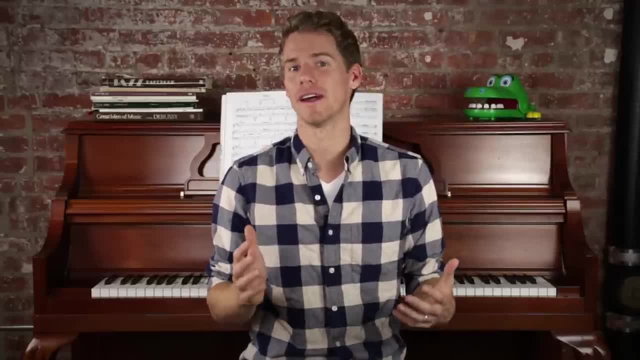 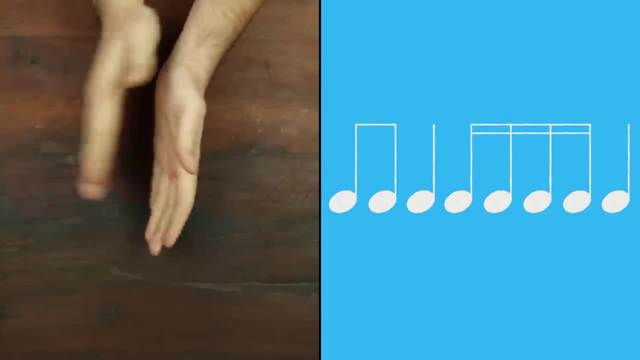 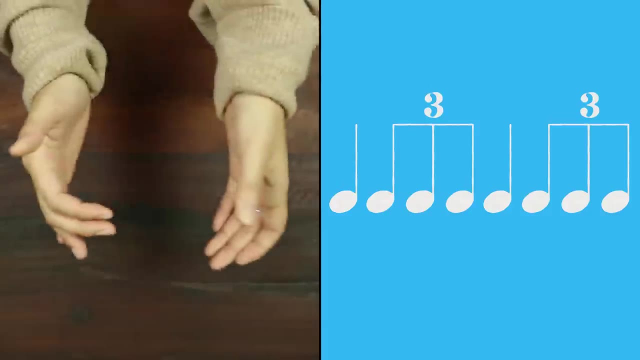 but track the beat by continuing to say one, two, three, four as I go. One, two, three, four, One and two, three and a four. One, two, three and four. One, two, triplet, three, four, triplet. 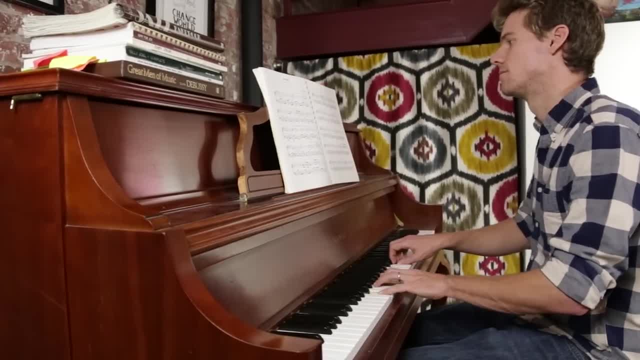 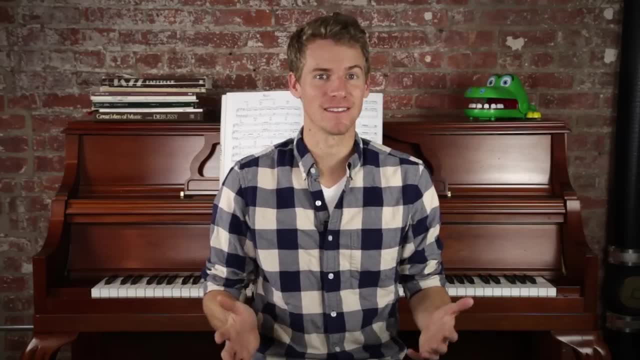 By figuring out the rhythm ahead of time, it's much easier to actually sit down at the piano and play the song. If you wanna get a little more fancy with clapping, you can tap the left and right hand parts on your knees. So I'll establish my left hand rhythm like this. 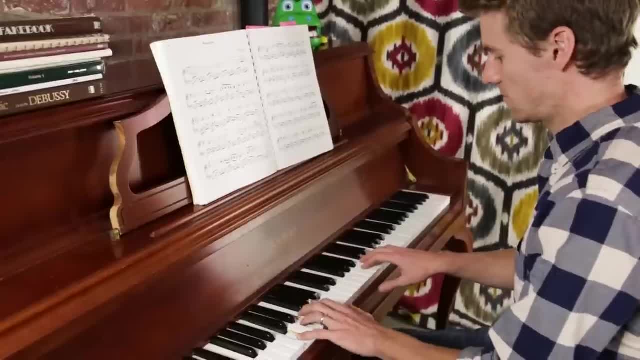 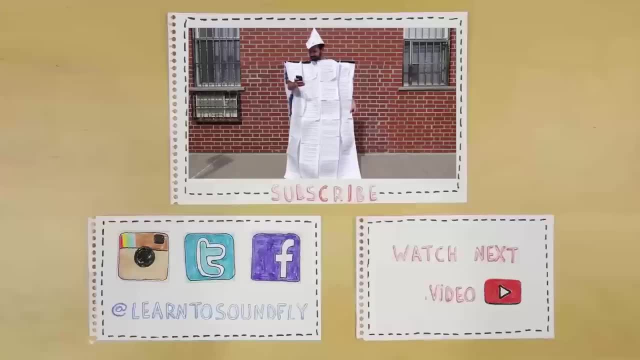 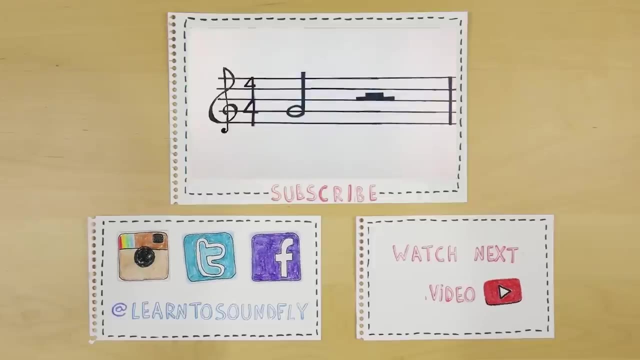 and then I'll add my right hand rhythm like this. This can start to get a little tricky, but it's a good way to practice different rhythms and start to get in the flow.